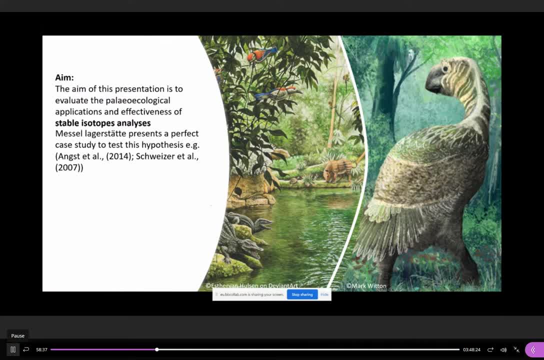 And the mesyl lagristatin presents a perfect case study to test this hypothesis, and it has actually been explored by previous authors. So the presentation is going to consist of two parts. In the first part I will dive into what approaches have been used in the past to reconstruct the food webs in mesyl. So how do we know? 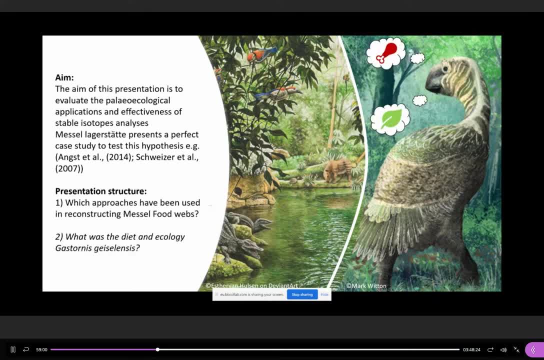 the relationship between the individual taxa And the second half of the presentation, we'll dive into the debate about the large so-called pterodactyl Gastonus which is found at this site and what its role in the ecology and its diet was. 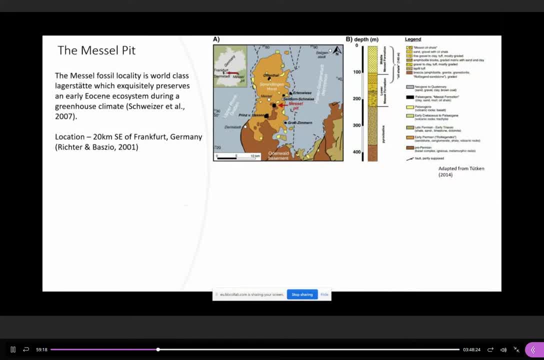 So to introduce the mesyl fossil locality, for those of you who don't know of it, it's a world-class mesyl lagristatin, which means a site of exceptional preservation, And it preserves an early Eocene ecosystem that was about during a greenhouse climate, And it's located in 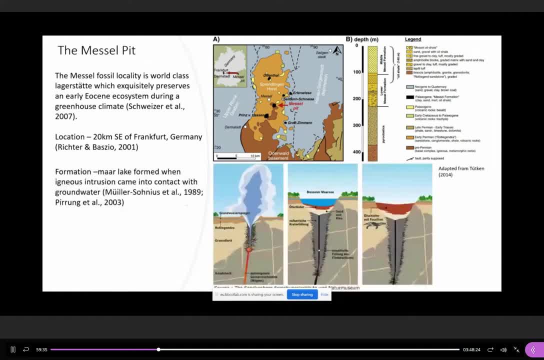 Germany, some 20 kilometres southeast of Frankfurt. The formation of the mesyl site is actually quite an interesting one from a geological point. It preserves a marl lake environment which actually formed when localised volcanic activity. an igneous intrusion caused the 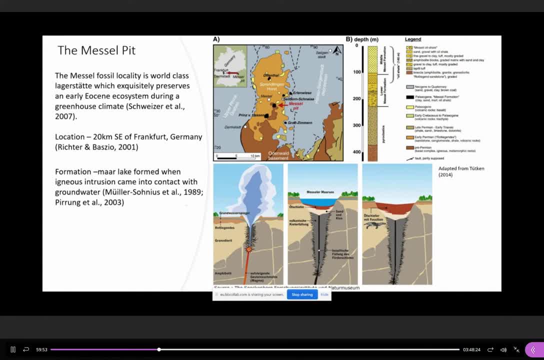 explosion, that's, molten rock came into contact with groundwater and that caused a lot of steam and generated a huge explosion which created this volcanic pipe and crater, which subsequently filled in and became a freshwater lake. The question of why so many fossil taxa. 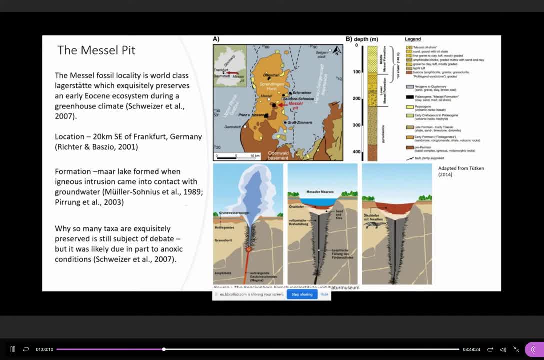 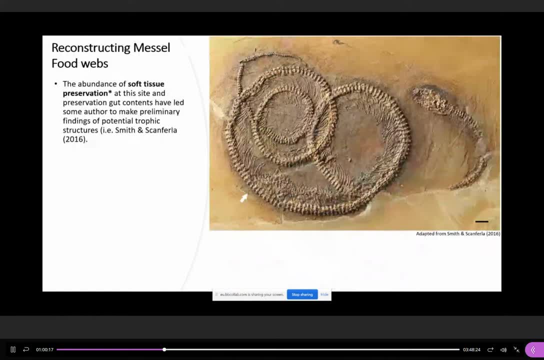 are so exquisitely preserved at mesyl is still a subject of current debate, and this is something we can return to in the questions. But it's likely due to, in part, anoxic conditions at the bottom of the lake. So how about research? 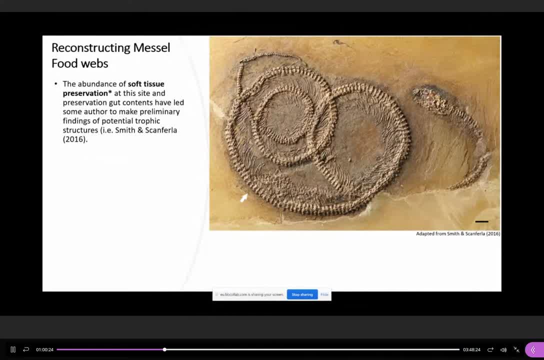 reconstructing the mesophid webs. So, as I just said, the mesocyte preserves is exquisite as it preserves soft tissue of the animals that were alive at the time, which is quite incredible. And you can actually see that here in this fossil snake, which is quite 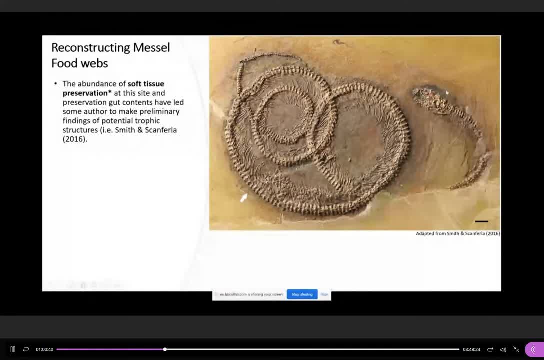 nice that we're going back to fossil snakes for a moment. there We can see the skeleton, but we can also see there's this dark shadow following around it, and that is original organic tissue that's been preserved And I think this being a vertebrate fossil. this 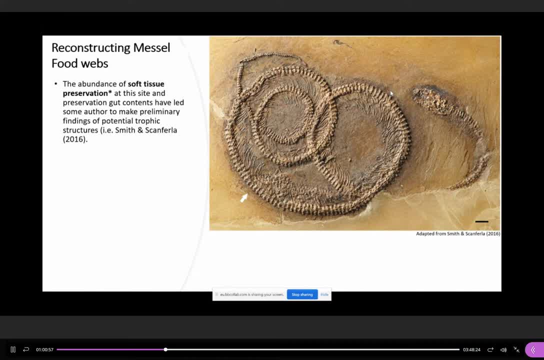 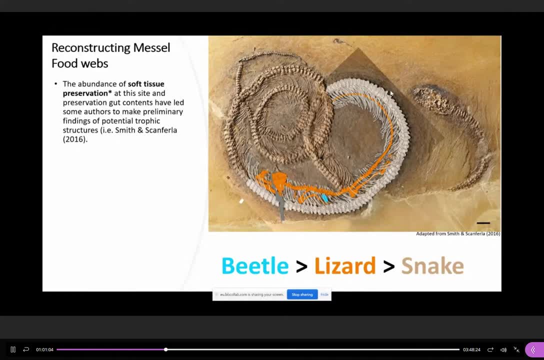 has to be probably one of my favourite vertebrate fossils, because we have inside this fossil snake a fossil lizard, and inside the fossil lizard we have a fossil beetle. So what this one fossil is actually showing is a potential trophic structure that the beetles were fed. 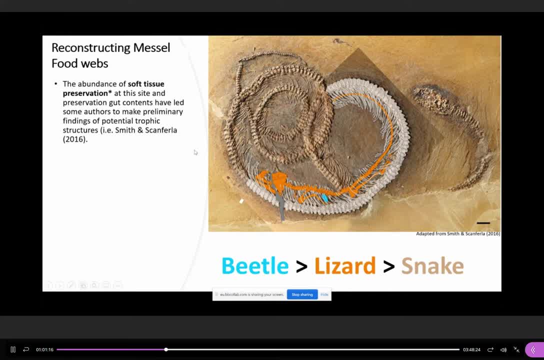 on by lizards, and lizards were fed on by snakes at Meso, which I think is incredible that we have this preserved, and this is what some authors have actually suggested. However, we need to be careful, because These rare, isolated discoveries risk to over simplify. 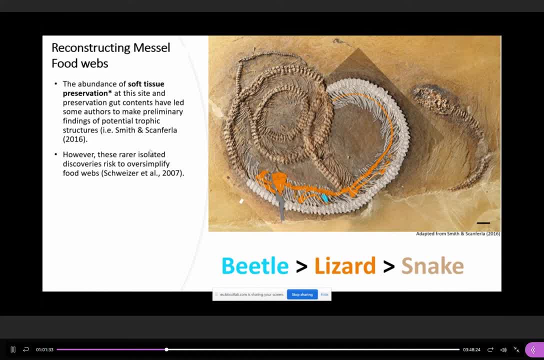 the food webs. We know that this snake, for example, fed on lizards and these lizards fed on at least some beetles, but we don't know if the snake or the lizards, for example, fed on other other other types of food sources. 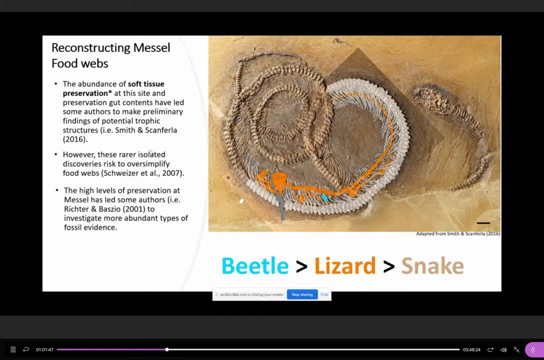 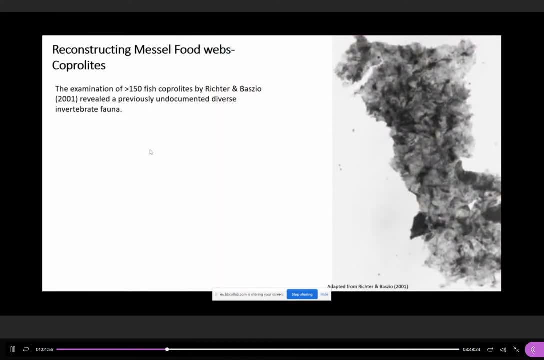 The High levels of The high levels of The high levels of fossil preservation at Messel have also led some authors to investigate more abundant types of fossil evidence, and they are less glamorous. they are coprolites. So a study done in 2001 by two authors examined over 150 fish coprolites from the ancient Messel. 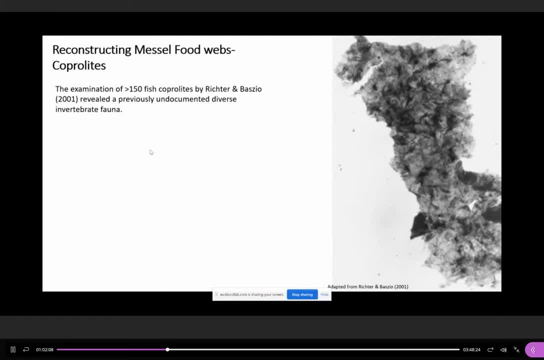 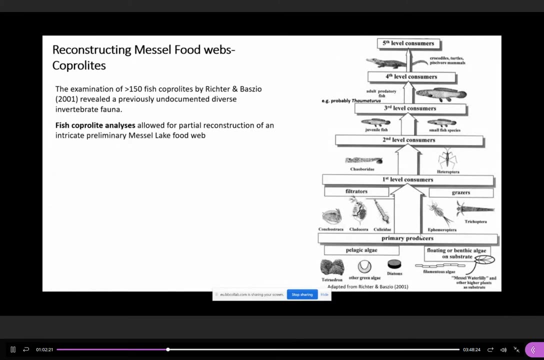 lake and actually revealed a previously undocumented and diverse invertebrate fauna, and we can actually see within this coprolite all these small fragments of insects and invertebrates And from this they were able to construct a simple food web and the advantages of doing. 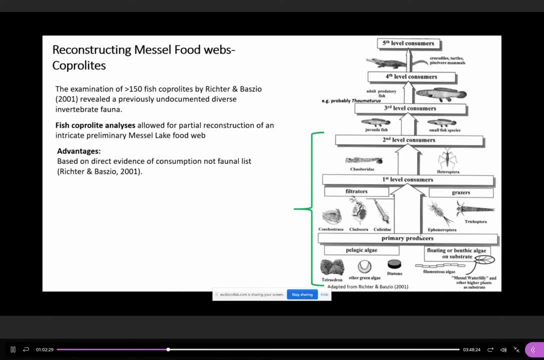 this is that we know that this is based on direct consumption. it's not just a faunal list that has been tiered, with the smallest animals at the bottom and the biggest at the top, and it also, in part, preserves this complexity of the Messel lake, which was 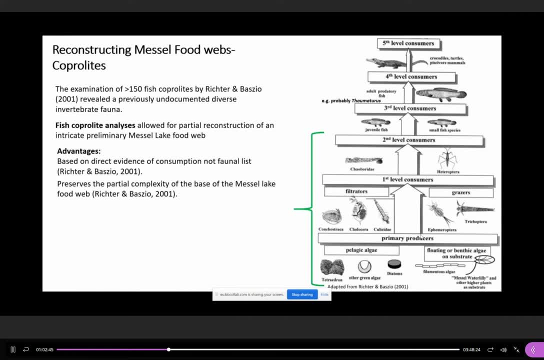 before then wasn't preserved. The large vertebrates are, but the smaller invertebrates were not. But there are disadvantages. The fish coprolites only preserve the lower trophic levels and not the higher ones. Also, there is talk about it being unquantitative. how can we quantify? 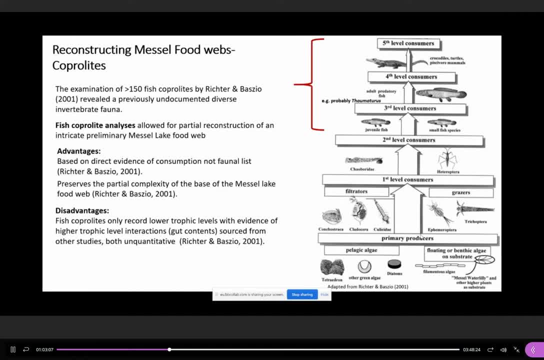 this with other sites and other parts of the locality. The difficulty, for example, is also shown by it's only really showing small fish what small fish ate. Everything above that is kind of left to speculation and the particular I've highlighted here, a particular genus of fish. 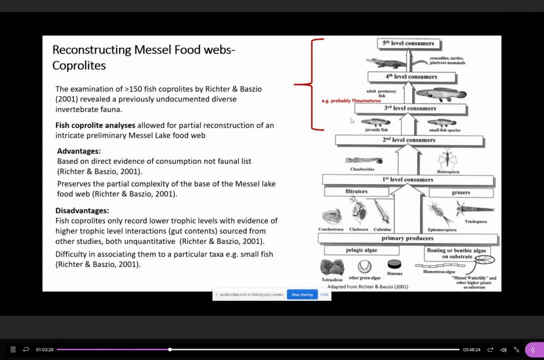 which we'll return to- which, in this diagram, has been placed as a fourth level consumer. But how can we be so certain about that? And also, to make matters worse, we have unintentional digestion. So these fish were swimming in the Messel lake and there was algal blooms and 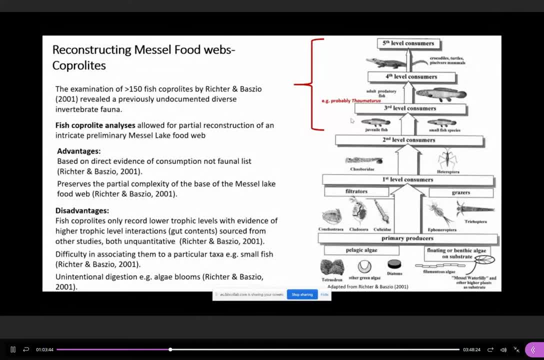 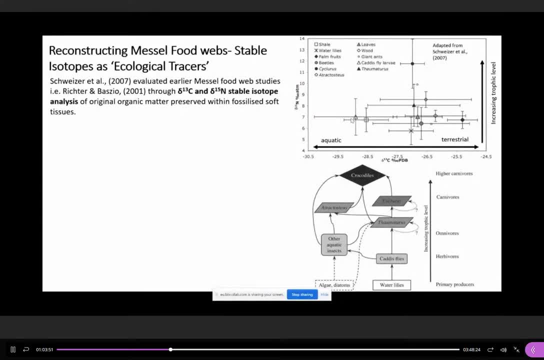 unintentionally they were swallowing these algaes, so it also just complicates the entire picture more. So what can isotopes do in helping us understand this a lot better? So a study six years later re-evaluated this earlier 2001 study through the scope of carbon-13. 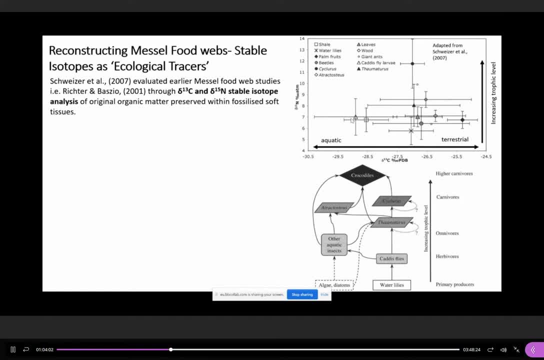 and nitrogen-15 stable isotope analysis- importantly on that original organic soft tissue that you saw on the snake just previously. So here the carbon-13 has been used as a proxy to distinguish between terrestrial and aquatic food sources. So if you look at this, 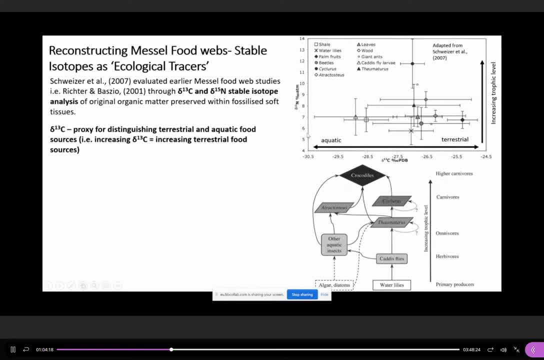 diagram in the top left-hand corner. as we get more negative carbon-13, we're more likely to be aquatic food sources, and as we get more positive carbon-13, it's more likely to be terrestrial. Nitrogen-15 isotopes have been used as a proxy to indicate the trophic position. 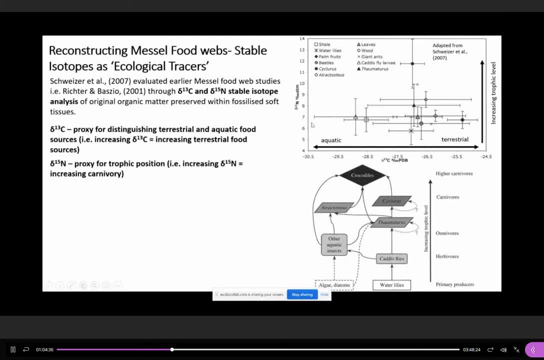 So things at the base of the food web should have a low nitrogen reading and as you progress up the trophic level towards the top of the food web, we should have higher nitrogen values, And the advantages of this is that actually these methods have actually been used in modern lake environments. 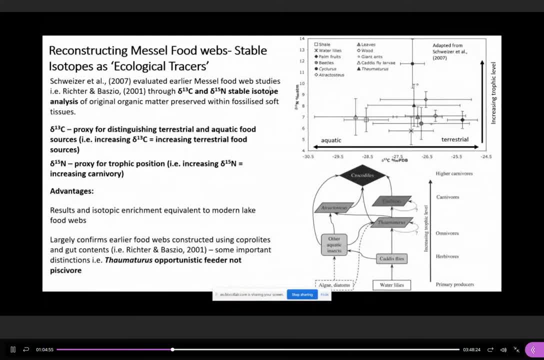 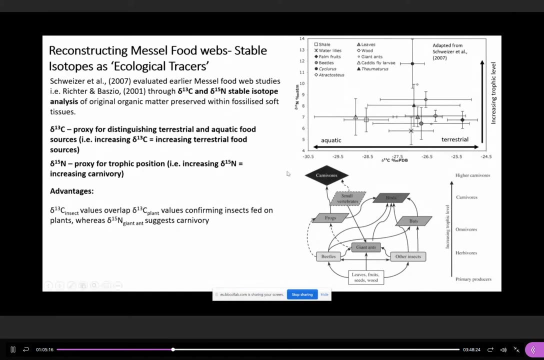 and the results are quite similar. It largely confirms these earlier unproven studies which looked at the coprolites and actually the fish. for example, has been now thought to be more of an opportunistic feeder rather than a full-fledged carnivore. Also, this particular diagram can distinguish between terrestrial 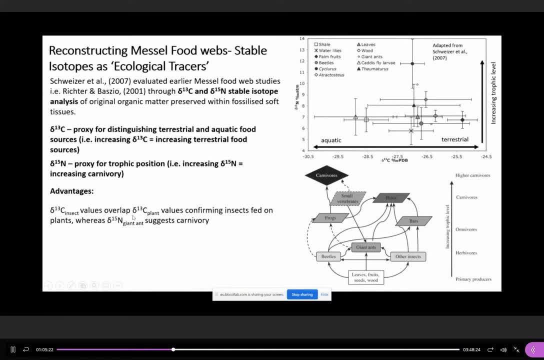 and aquatic food webs. So, for instance, the carbon-13 measurements within insects that were analysed overlap with carbon-13 measurements in the plants, confirming the insects indeed fed in plants. But interestingly, some insects, like the giant ants, had the nitrogen-15 values. 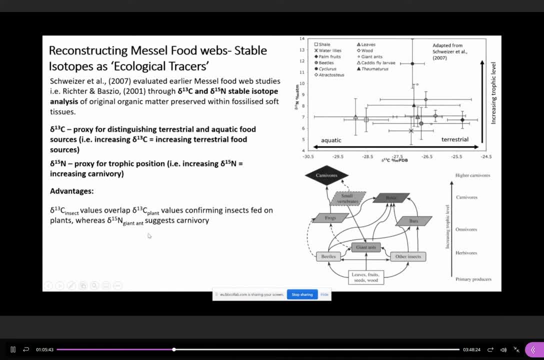 higher than other insects, suggesting carnivorous. So this is a very interesting diagram And this is a very interesting study. So there's these giant carnivorous ants at Mesa, which is quite interesting. We also see again increased nitrogen-15 values in taxa, such as crocodiles. 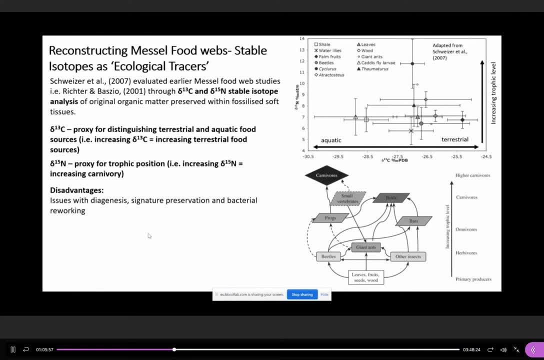 and other larger invertebrates. There are disadvantages with this technique- potentially diagenesis and other sorts of environmental factors that can influence the signal- And it seems that this can't be used on its own. We need to use this along with the other species. So it's not an easy task to do. We need to. 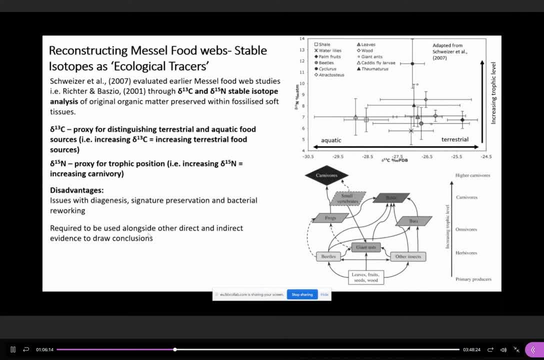 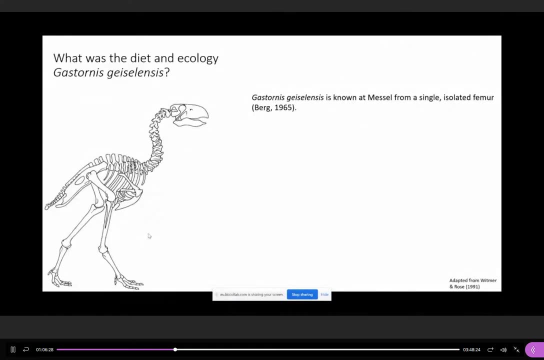 alongside other direct and indirect paleontological evidence, to really draw some firm conclusions on the structure of the food webs. And also, this was a first of its kind study, but larger sample sizes would be needed to do in the future. So quickly moving on to part two: what was the diet and ecology of this giant pteroduck? 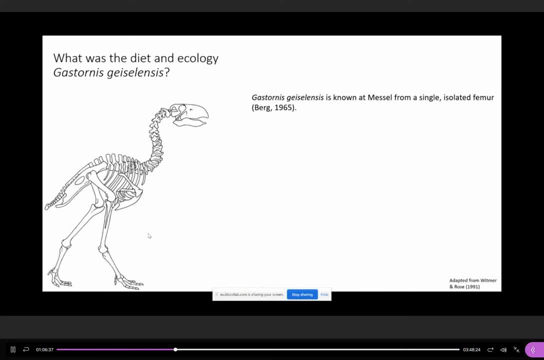 as it's called, Gastonus. So this Gastonus species is actually being discovered at Messel from a single isolated female back in 1965. But it was originally described from early paleogene of France in the early 1850s And the notorious American paleontologist Edward 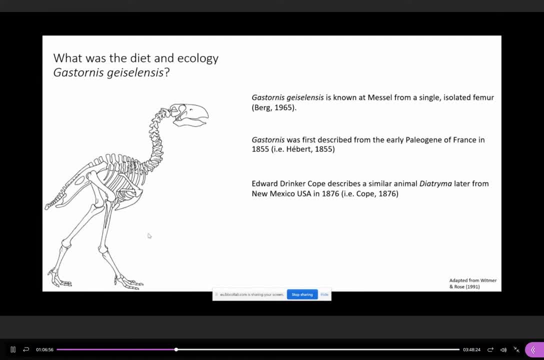 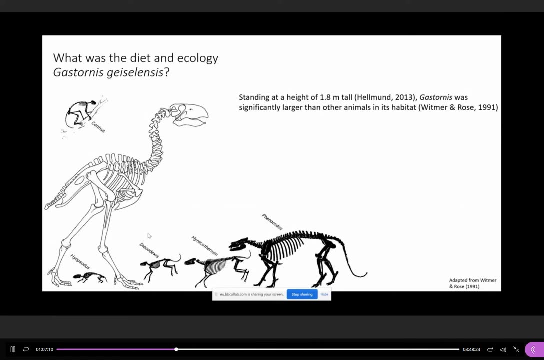 Juncker Cope actually described a similar animal, diatryma, from New Mexico, 20 years later, But we now consider that Gastonus and diatryma are actually considered the same taxon, So this was a big animal, Standing at about 1.8 metres tall. Gastonus would have dwarfed all other animals within. 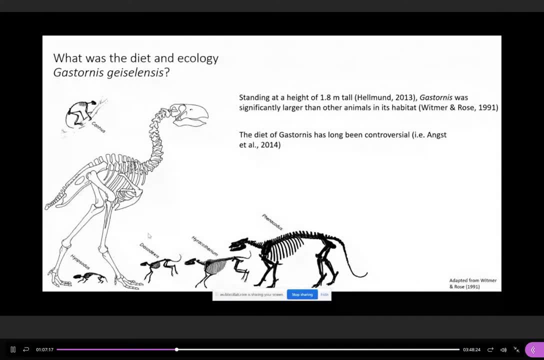 its ecosystem in the early Eocene, And this has led some potential authors to question the diet of Gastonus. Potentially was this a huge hyper carnivore that was preying on our early mammalian ancestors, Or perhaps as simple as that And although a nut cracking. 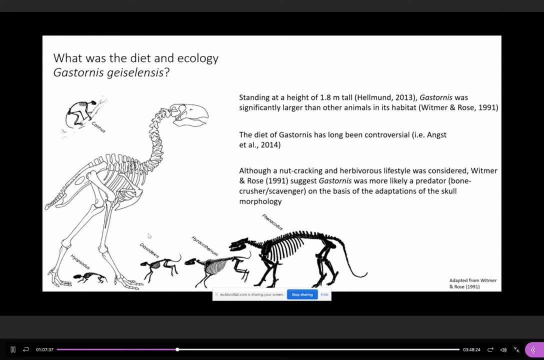 or herbivorous lifestyle has been considered. Whitmer and Rose in 1991 suggest that Gastonus was more likely to be a male than a female. But the diet of Gastonus is not the only thing to be a predator, specialising potentially in bone fishing or scavenging on the basis. 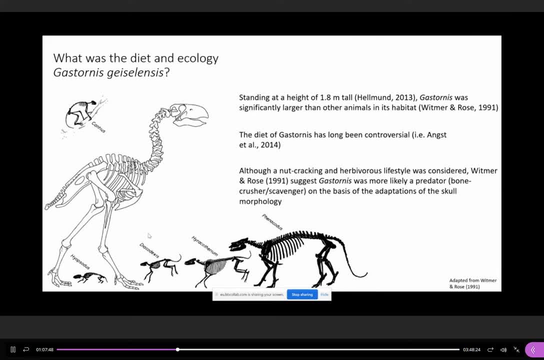 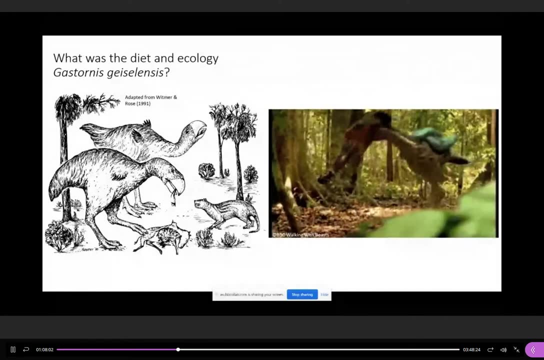 of the adaptations of the skull morphology. Its skull was so large and reinforced. these authors just couldn't see why it would be a herbivore. This had to be a carnivore And this interpretation had lasted. You might remember the BBC Walking with Beasts trilogy. 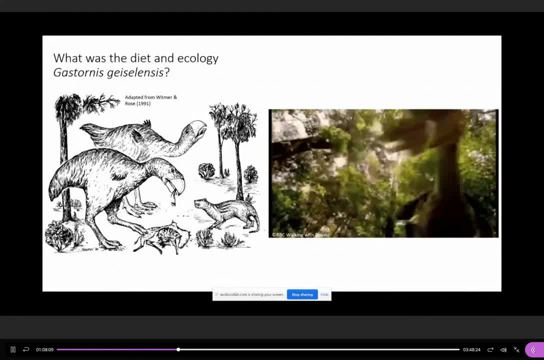 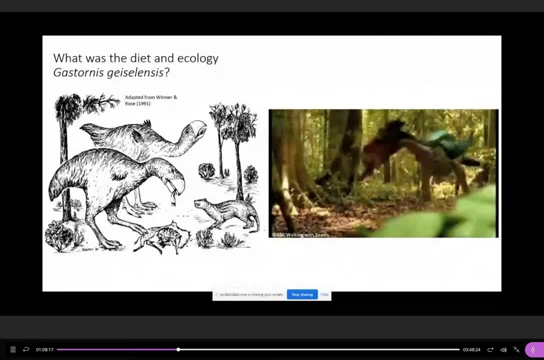 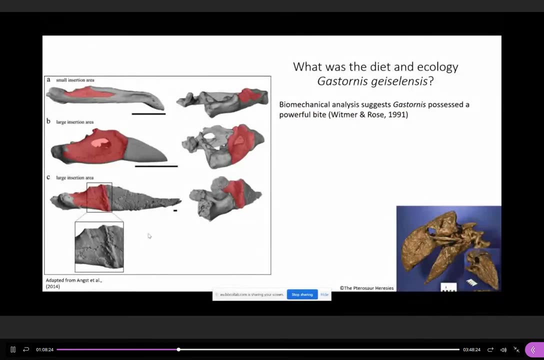 back in the 90s, And popular media now portray these large birds as active carnivores preying on these small horses. But how accurate is this interpretation? Whitmer and Rose did do a biochemical analysis on Gastonus and it showed that it did have. 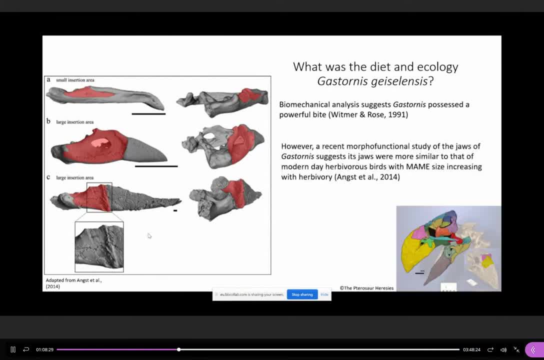 a very powerful bite. However, a more recent morpho-functional study on the jaws of Gastonus have suggested that the position of the muscle scars on the skull was perhaps due to the natural appearance of the animal on the skull which you can see here would correlate with: 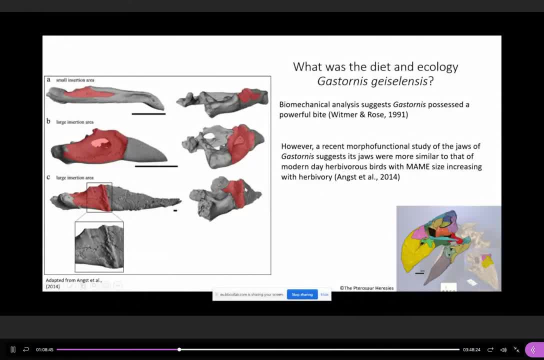 which are called mame, correlate. the size of these muscles actually correlate with herbivory. So carnivorous buds, modern day buds, have small muscles, whereas larger buds that break nuts, for example, have larger muscles, And this is something we see in Gastona. 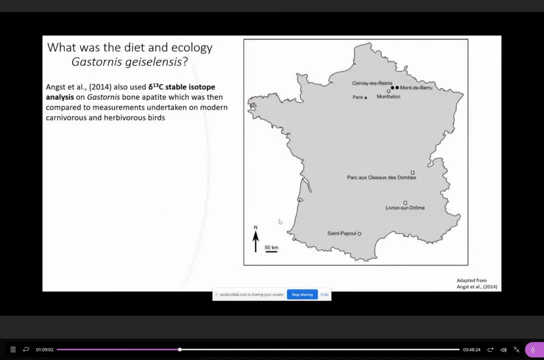 So potentially it could have been a helbivore. So how do we prove this? So again we come back to isotopes, and the same study that suggested this also employed again carbon-13 stable isotope analysis in Gastona's bone appetite. 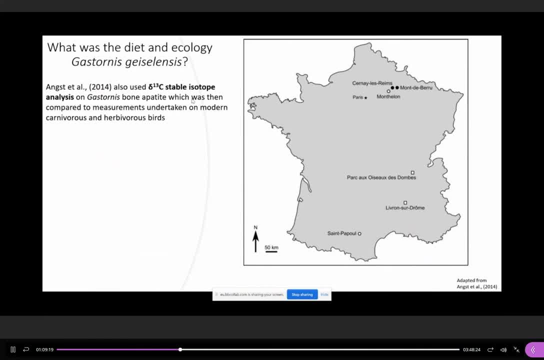 which was then compared to measurements taken on carnivorous and herbivorous buds from the modern day. This time, carbon-13 was a proxy for diet, So decreasing carbon-13 would relate to increasing herbivory, And the advantages of this is that the Gastona's material was sampled. 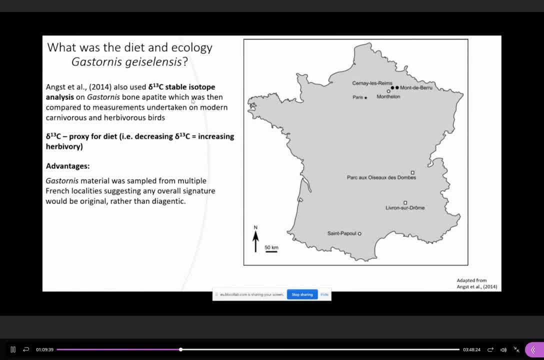 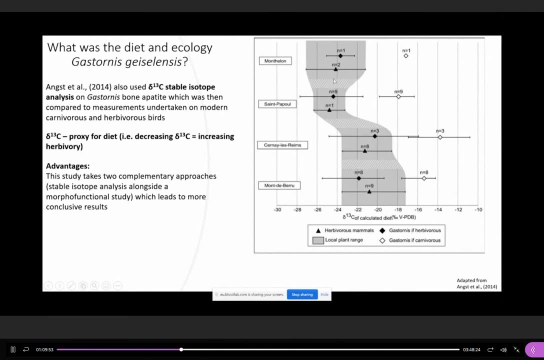 from a multitude of different branch localities, So this could limit the overall signature. if an overall signature was produced, this would suggest maybe a more original signal rather than a diagenetic one. And this is the actual graph here and we can see.